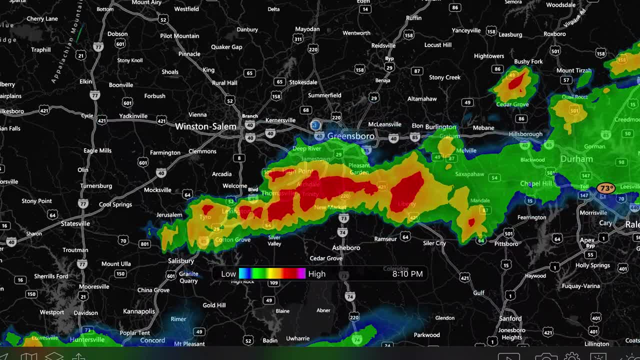 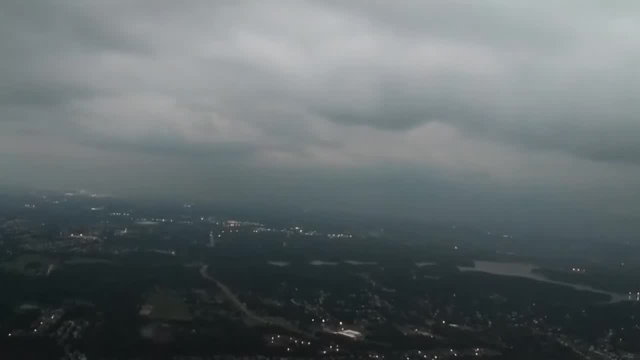 GSO Greensboro, North Carolina, and it's also backed up with what we see here on our iPad on a weather app showing a storm approaching the airport from the southeast. Now, as the aircraft descends below the clouds, obviously it's going to get a little darker, because now we're below. 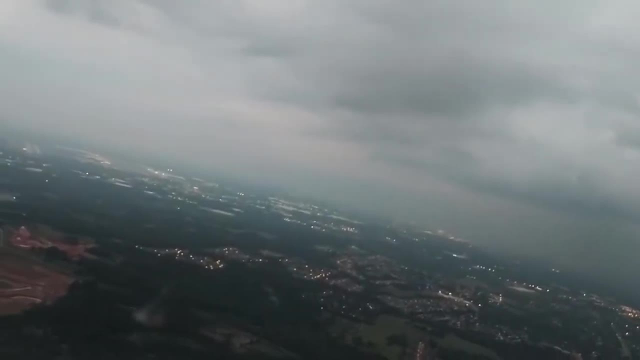 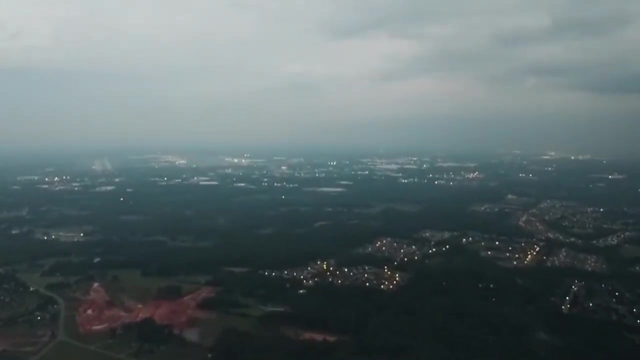 the clouds. there's lots of moisture, lots of water in those clouds blocking out the sunlight, and it's approaching evening time as well. This is getting close to 8 pm, eastern time. As the aircraft is on approach, we can see some lightning. 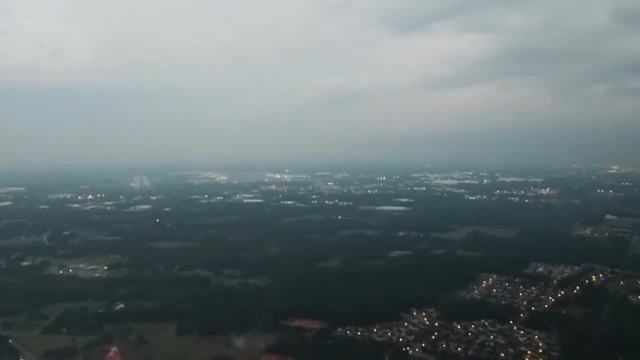 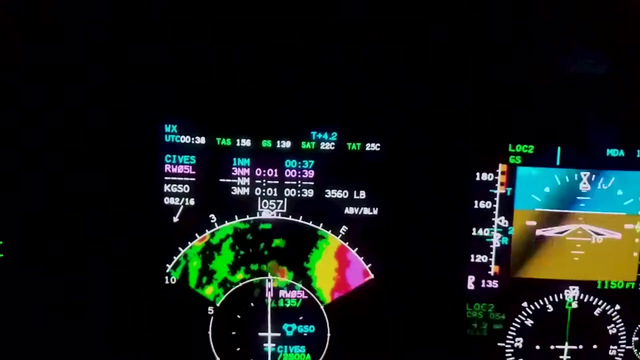 flashes off the right as they're approaching to land on runway 5 left and we can see those radar returns from the onboard weather radar on the aircraft, showing the storm still off their right. a good reason: they're landing on runway 5 left. Now there's something very important to note here. 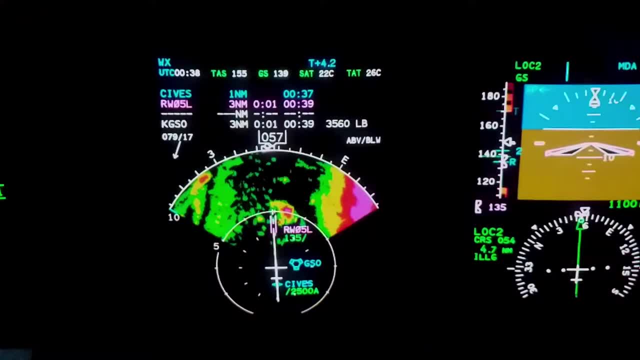 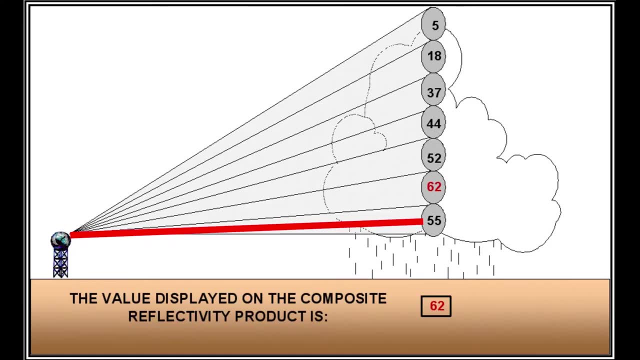 about the onboard weather radar. Notice the tilt is at plus 4.2 degrees, very similar to how the tilt works on the radar ground stations where they take several scans of the sky at different tilt angles and then compile those images into the radar. 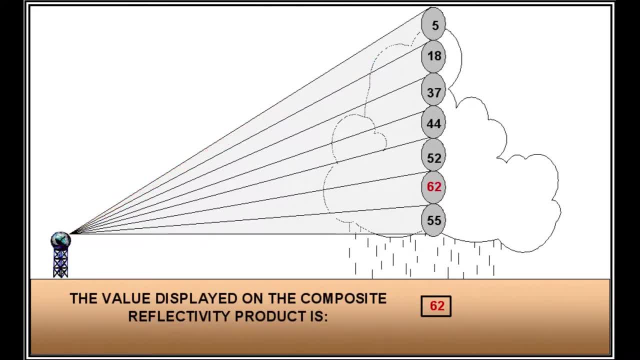 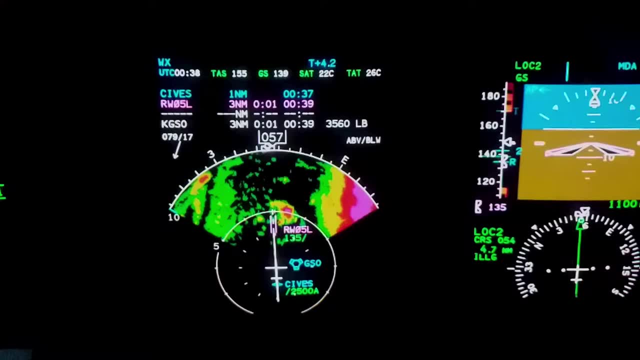 We know that takes about 4 to 11 minutes to occur and that's not good when you're in an aircraft that's moving 6,, 8, 10 miles in a minute in these really high-speed jets. That is why the tilt is specified. 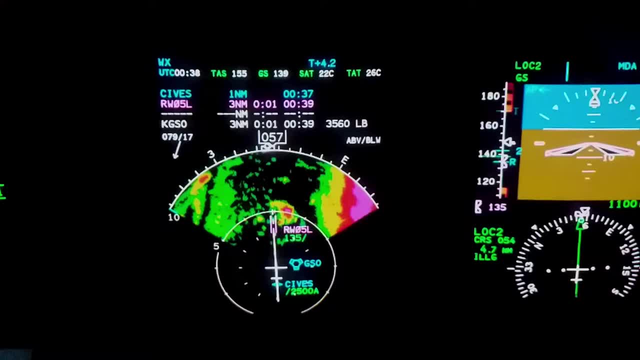 right at 4.2 degrees and is not moving up or down. It's simply scanning that one slice of sky just to grab the image and give you the immediate information there. So it's up to the pilot to control the tilt here. It's not making a composite image of several tilts as a ground station would. 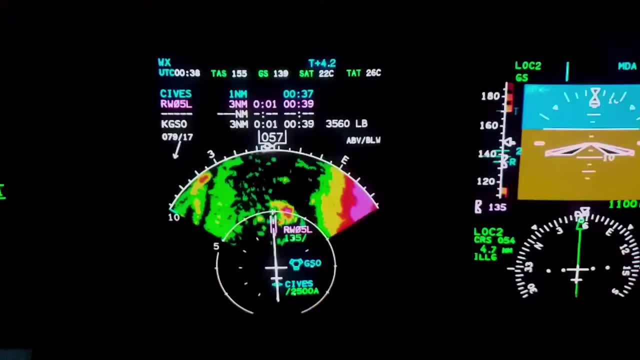 it's simply looking at one slice of sky. Of course, if the pilot tilts it too far down, you may wind up with some ground clutter, as you do here. And then when you see very large returns, like we do here on the right, obviously that's going to have to be some sort of mountain. 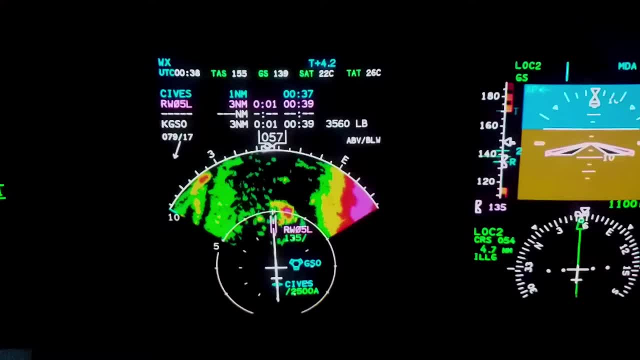 some sort of large terrain or in this case, it is in fact a very large thunderstorm with lots of water in it. Now, as soon as this aircraft landed, there's so much lightning in the area that they were stuck out waiting for people to come from the FBO to guide them in. 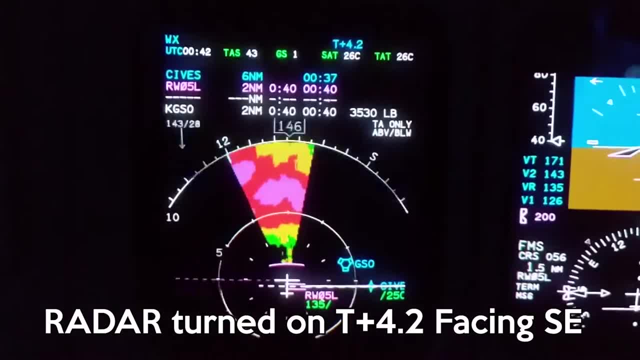 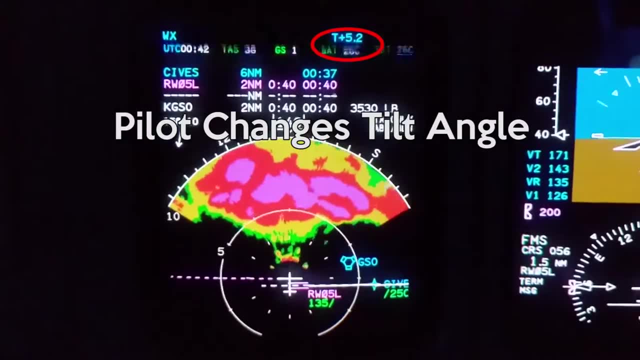 And so that's why it's so important that you pay attention to the radar on the onboard weather radar, as it's very important that you watch out the window as the storm moves over, as well as looking at what the onboard weather radar is showing us here. while they're on the ground, It still works while 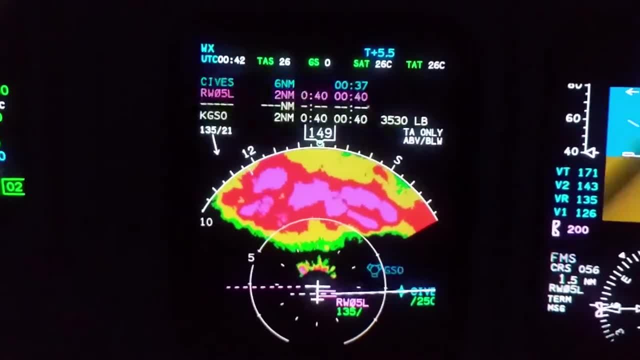 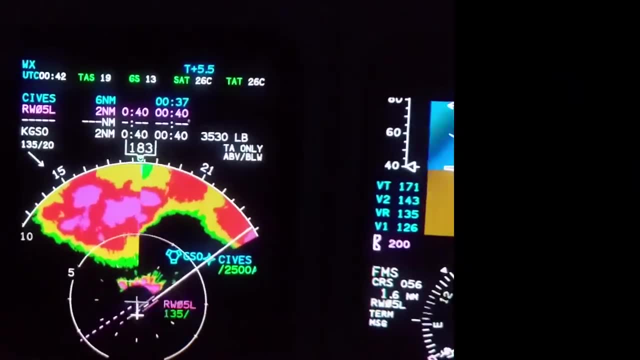 they're on the ground. They obviously just have to tilt it up high enough that they're not getting too much ground clutter or too much interference from anything that's above the nose of the aircraft where the radar is located. We can compare what we see on the onboard weather radar to what 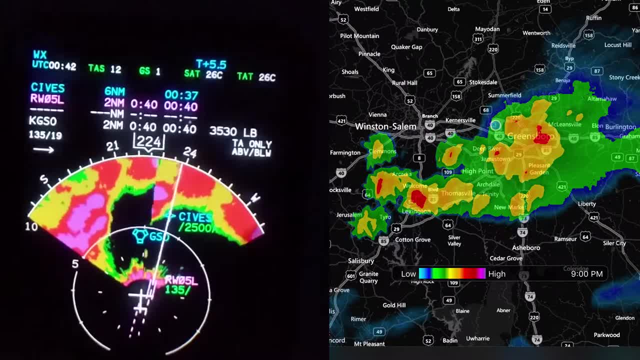 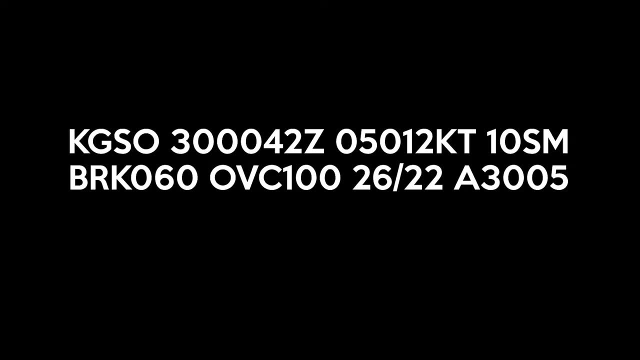 we see on the iPad, just using the internet as a connection to see the radar images that are being. that's then sent to us via the internet on our iPads or cell phones, And we can also compare the METAR at the time the aircraft landed. 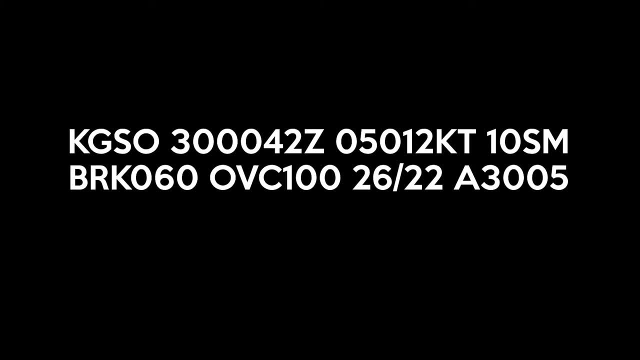 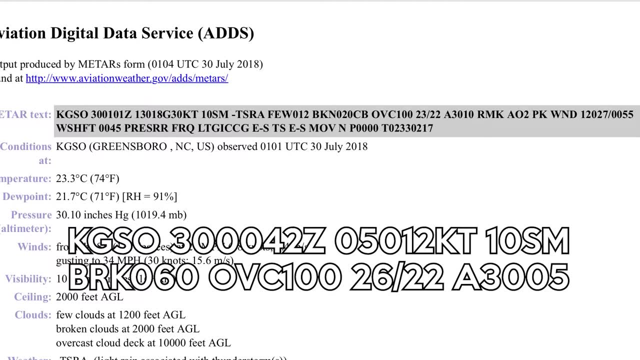 to the updated METAR just about 15 minutes later, when another aircraft had come in on final and reported a 20 knot gain of airspeed on final. So a large increase in performance. That's a huge warning sign that you may get that decrease in performance. 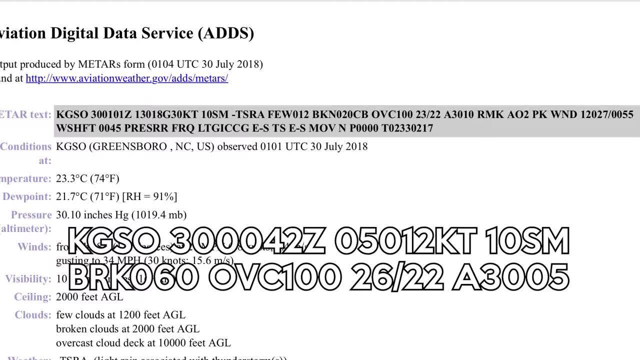 And gaining 20 knots is not good, but losing 20 knots, of course, is even worse. That aircraft was able to land safely, But look at how the METAR changes between these two times. So we have the time that the first aircraft landed. 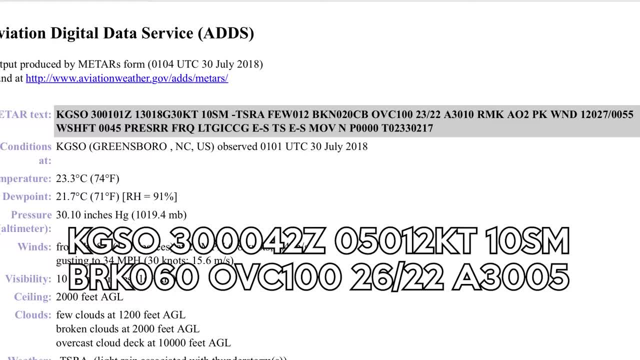 And then, just 15 minutes later, as the storm is getting closer and closer to the field, we get the gust front that comes out of that thunderstorm, As all that water is falling down, all that cold air is falling down, it hits the ground in a one large giant downdraft. 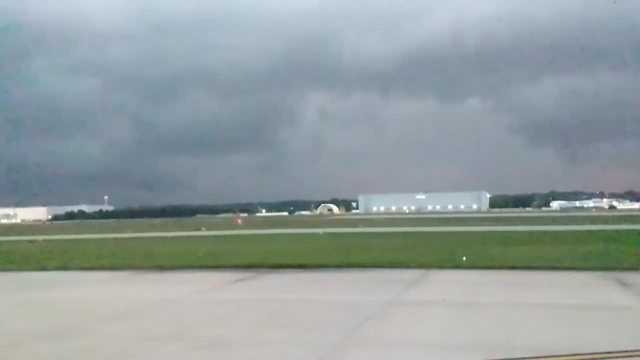 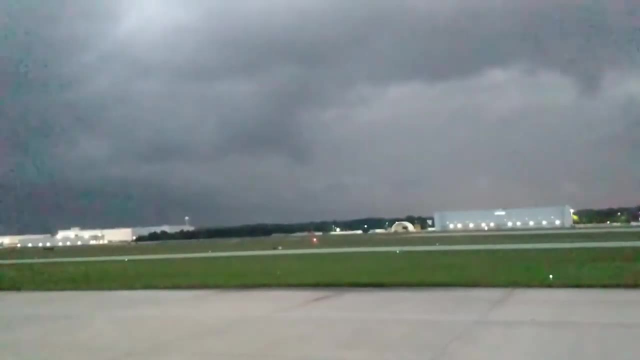 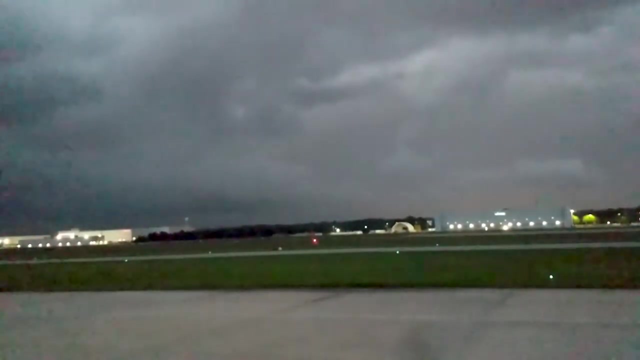 and then has to go somewhere and it turns into horizontal wind that causes very severe wind shear on takeoff and landing, as well as just very strong surface wind around the airport in general. A good takeaway from this video is, although the radar imagery on the aircraft itself is just a single tilt angle, it's instantaneous. 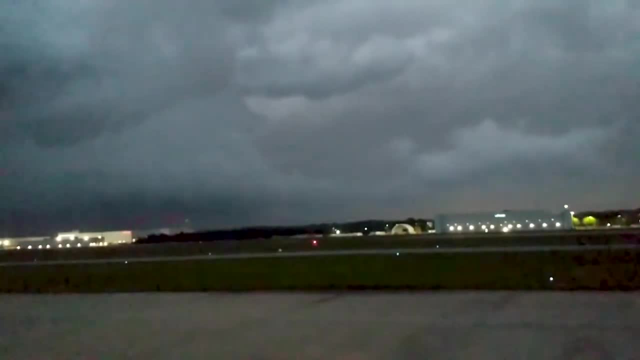 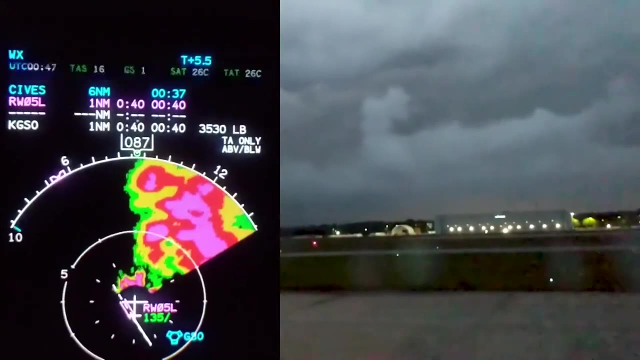 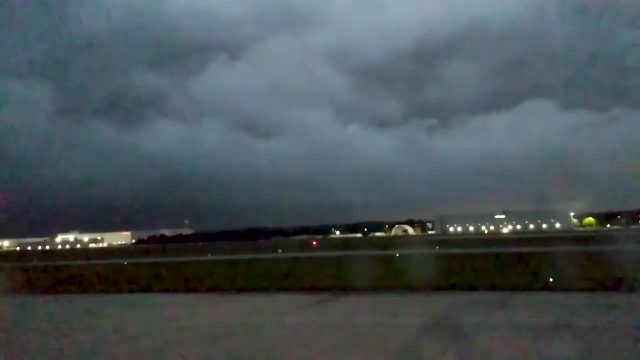 Almost only takes a few seconds for that radar to scan and then display that information to the pilot of that one slice of sky, compared to the ground stations taking perhaps a more accurate or more complete image of the sky with several scans at different angles. However, it takes much longer, four to 11 minutes for those ground. 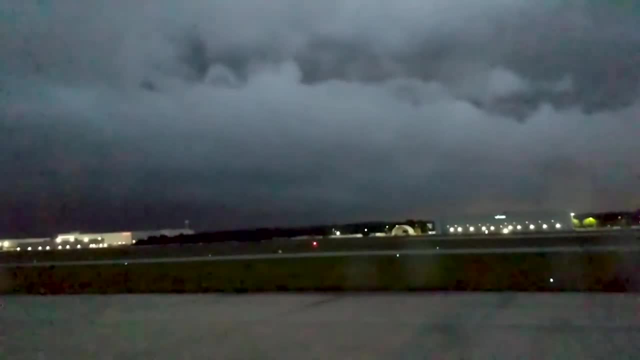 stations, to compile all that data and then make an image and then for it to actually go out to separate weather providers. that will make it through to your cell phone or your iPad through an app such as this and then come to you So you could be looking at data that's easily 15 or 20 minutes old.